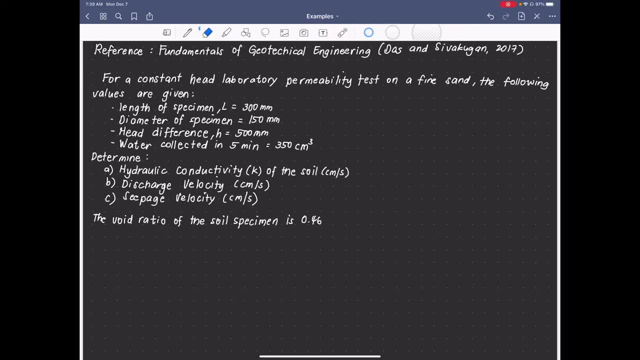 using a constant head laboratory permeability test. For this test, the following data are obtained or data are given We have: the length of the specimen L is equal to 300 millimeter. The diameter of the specimen is 150.. The head different age is 500 mm. The water collected in 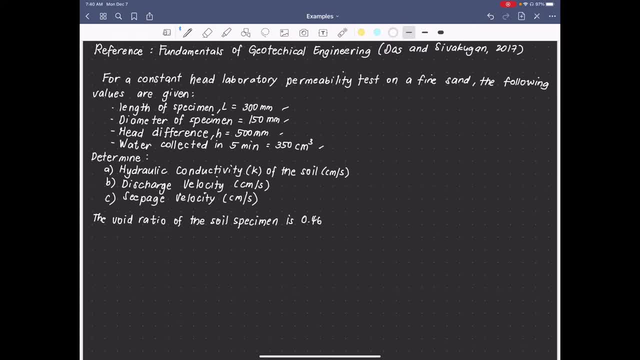 five minutes is 100 milliliters. The diameter of the specimen is 150.. The head different age is equivalent to 350 cubic centimeter. For this test, we are asked to determine the following: The hydraulic conductivity of the soil in centimeter per seconds. The discharge velocity. 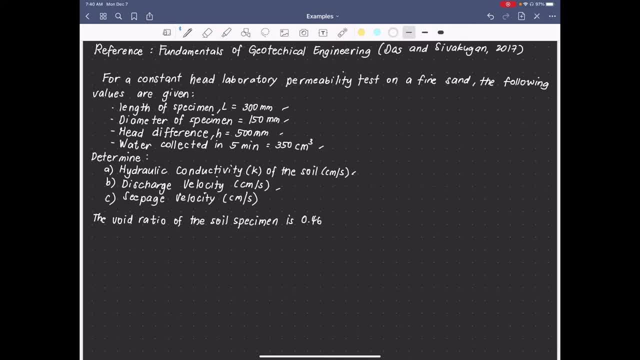 in centimeter per seconds also, and the seepage velocity with the same unit. The void ratio of the soil is also given to be 46. So in the constant head test we are using a permeability test under a constant head difference. So let's try to draw. 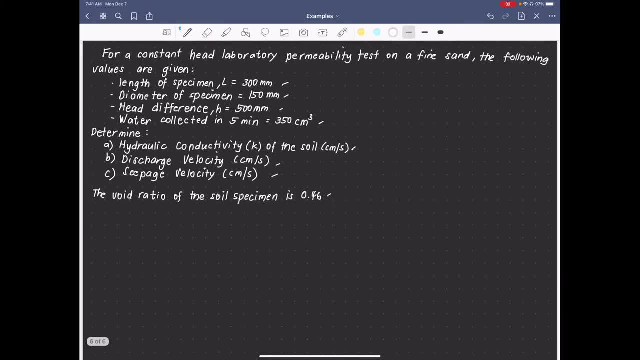 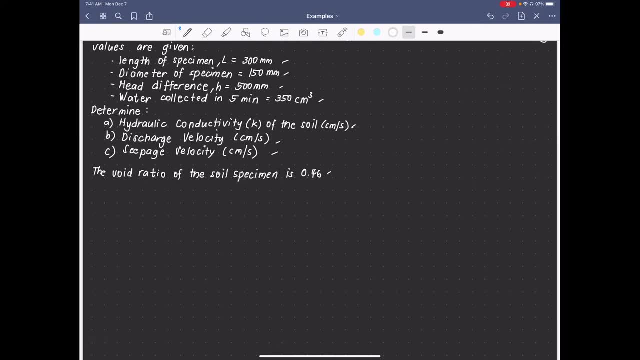 the soil sample and the permeability apparatus. So we are given a permeability apparatus, let's say this one, And the consequences are these. So for these samples, if an imp Alexa gave the sample link and feed from another and I alreadysized the sample out for it to be은 number of times, Okay. 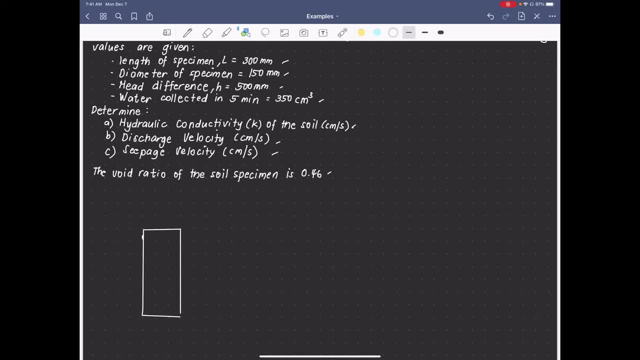 If the Dyos is not related to this sample, you will have to use the afterwards or a default samplingisión, And you can see that for any of these samples you would have to use the after muscles, so you'd have to use your formal form as your buffer for the selection. 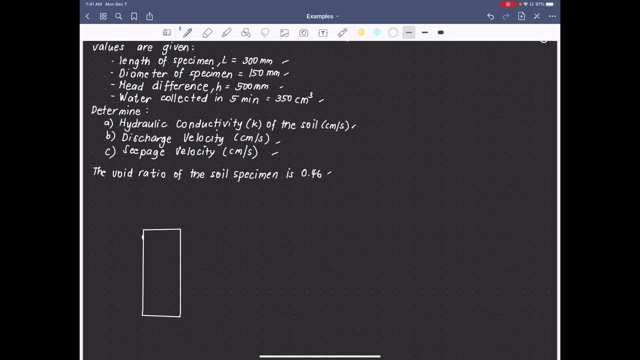 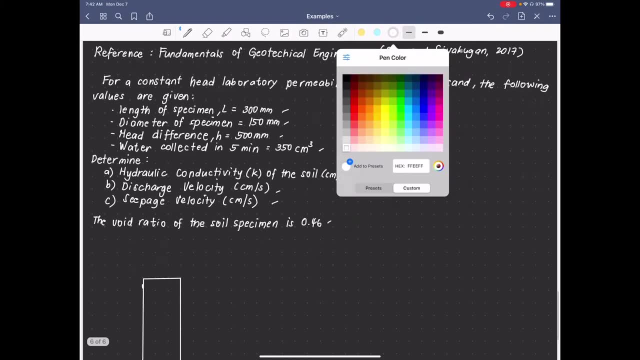 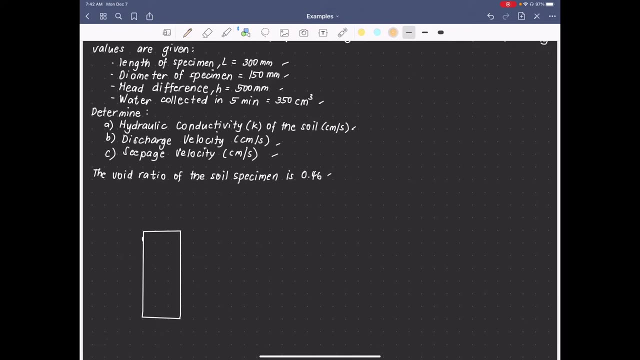 Okay, so this is the permeability apparatus. and then our soil sample is, say here and here, So this is the fine sand Having a length of 300 mm, or say this is 30 cm, okay, normally prior to the fine son we put: okay, we put porous stone on top and at the bottom, okay, so this is the porous. 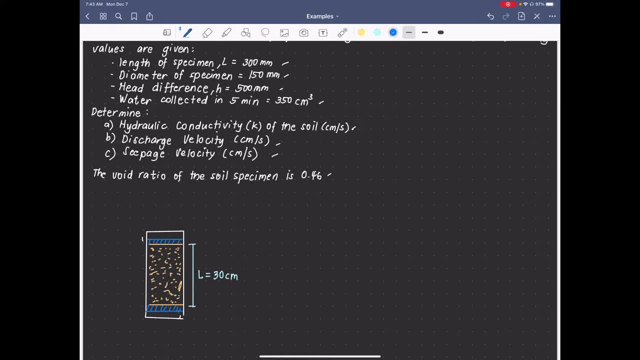 stone and the diameter of the specimen is 150, so there's no problem with that and we have a the head difference. so to get the head difference, what we normally do for this test is we allow water to flow through the permeability apparatus. oh, sorry to. 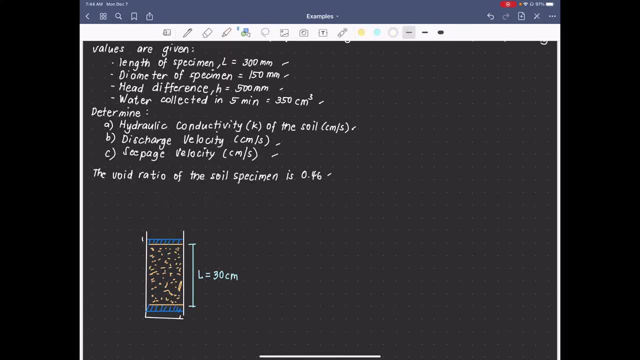 the permeability apparatus through a certain opening. okay, all right, this is connected to a funnel and this funnel will have a discharge here or an overflow. we call it an overflow better, so that when we allow water from the faucet to get in, water will flow here through our soil sample. but having 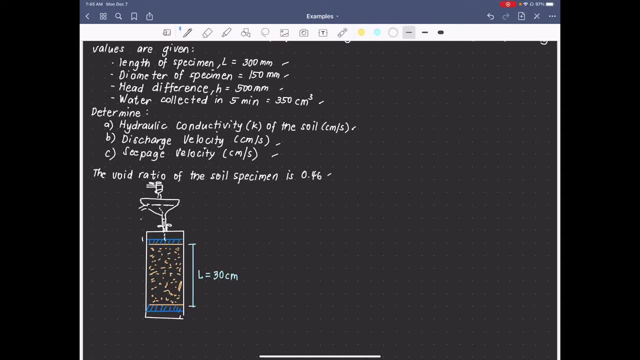 a constant level. only there should be an overflow here, so that the water will just have a constant level here, and once the water flows in our sample, we'll have two go out to our outflow, say here, and then water will be in a graduated cylinder. okay, so here and so the distance from our inflow, the 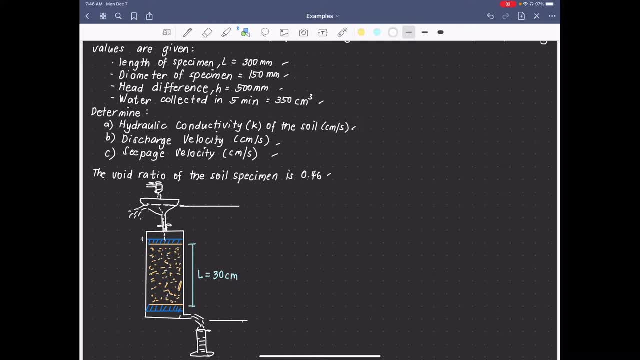 outflow will be our head difference, and that would be our H. this is our H, which is equivalent to 500 millimeter or 50 cm. so here the collected water is our H Q, which is 350 cubic cm, cubic centimeter. okay, so we need the hydraulic. 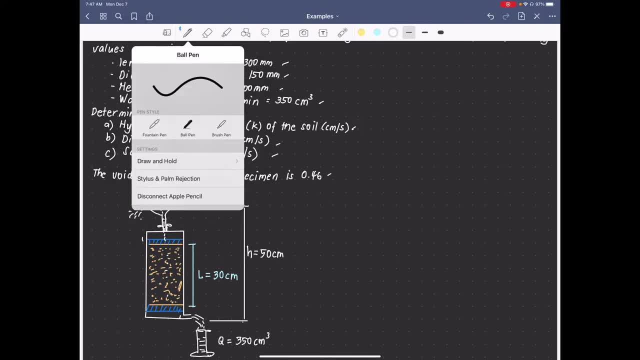 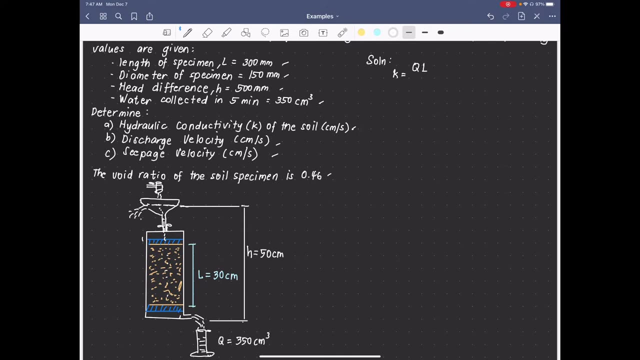 conductivity K, and we have a formula for that: the hydraulic conductivity is H, given to be Q by L, divided by A, by H by T, where in Q is the discharge or the total amount of water collected at a certain period of time. in our case it is: 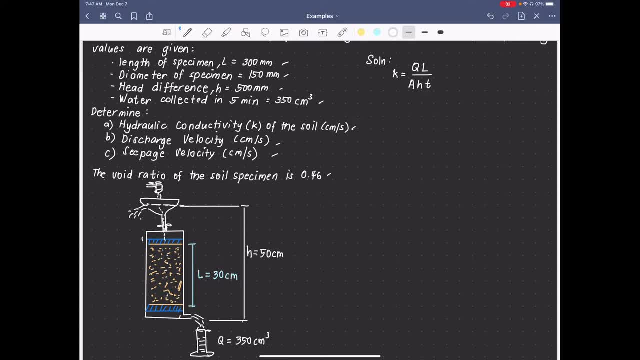 5 minutes. length: l is the length of the specimen, which is 30, and area is the area of our soil specimen. area is the area of our soil specimen. The diameter is given so we can compute for the area. H is the head difference and T is the time for the collection. 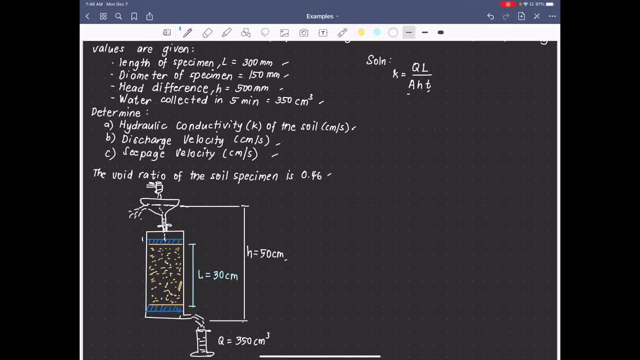 So all data are given so we can just plug in the values. Take note that we need the hydraulic conductivity in centimeter per second, so we have to convert some of the given values. Q is 350, that's already in cm, so this is cm cubed. 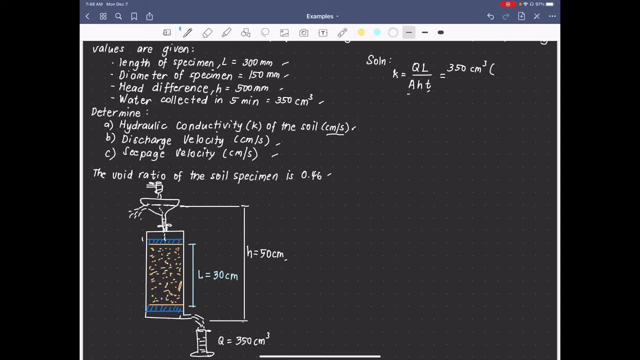 The length of the specimen is 30, this is in cm centimeter all over The area of the specimen. that is cylinder. our permeability apparatus or permeameter, is a cylinder, so the area would be, let's say, 5 or 4 times D, or the diameter is 150 millimeter. 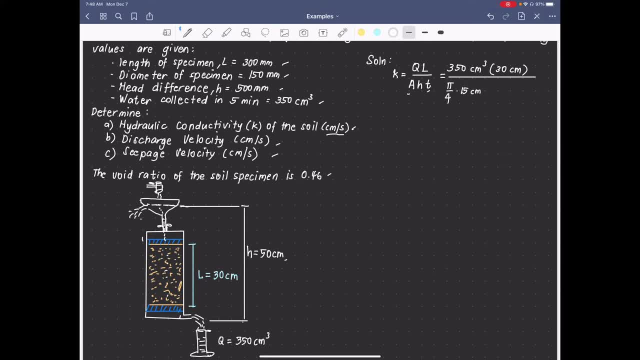 and that would be equal to 15 cm squared, and this is a square also. Then we have the head difference of 50 cm, so this is 50.. And the time required to collect the total amount of 350 is 5 minutes. 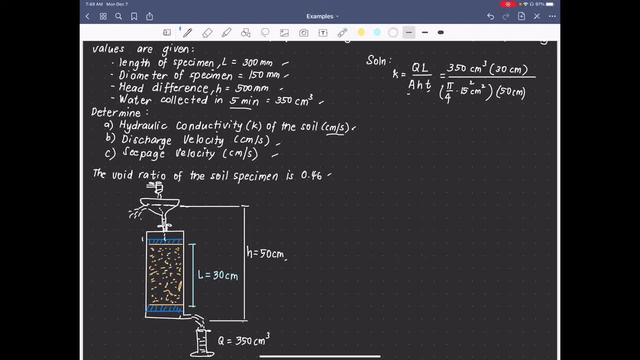 Or that is equivalent to time 60.. Let's make it in seconds, because we need the permeability in seconds. So 5 minutes is equivalent to 300 seconds. Okay, Okay. So the resulting unit would be centimeter per seconds. Calculating the permeability, we will get 3.96. 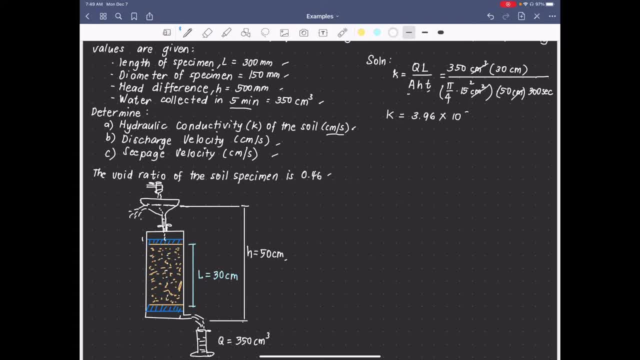 raised to 10, negative 3 centimeter per seconds. So this is the answer For letter A. normally for sand, the value is in the range of 10 to the negative 3, to the negative 2, up to negative 4.. 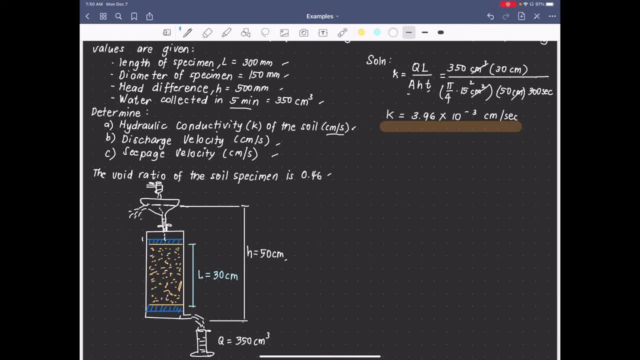 Then we have for letter B. we need to solve for the discharge velocity. Okay, The formula for the discharge velocity is equivalent to hydraulic conductivity by I or the hydraulic gradient, And hydraulic gradient is equivalent to the head difference divided by the length of the specimen. 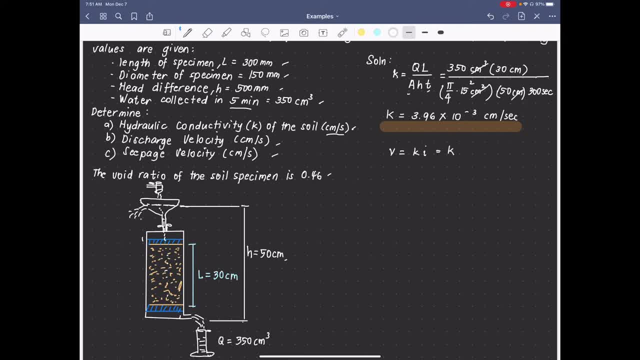 or this is equal to K multiplied by H over L. So here we have 3.6.. 96 times 10 to the negative, 3 cm per seconds multiplied by our H is 50. cm divided by L of the length of the specimen is 30.. 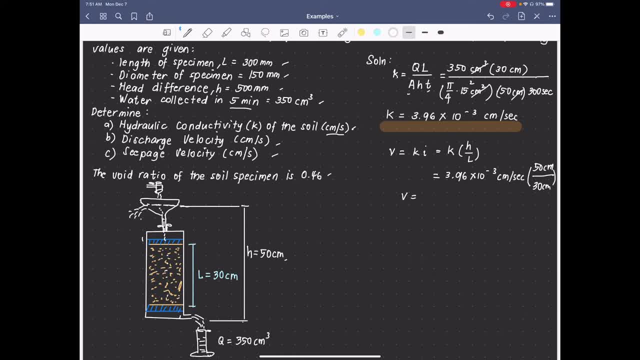 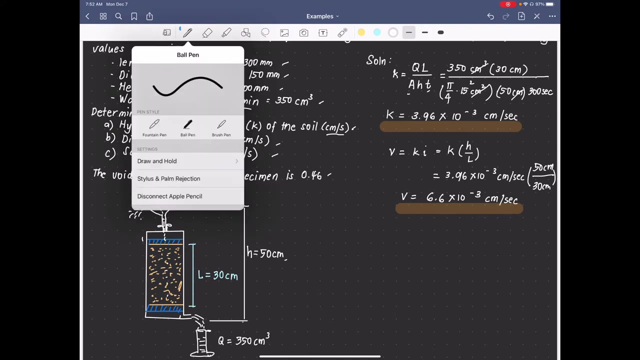 Okay, Okay, So V or the discharge velocity would be equal to 6.6 times 10, to the negative 3 cm per seconds. Okay, Then the sippage velocity is denoted as V sub S And the I or the discharge velocity is equal to 6.6 times 10, to the negative 3 cm per second. 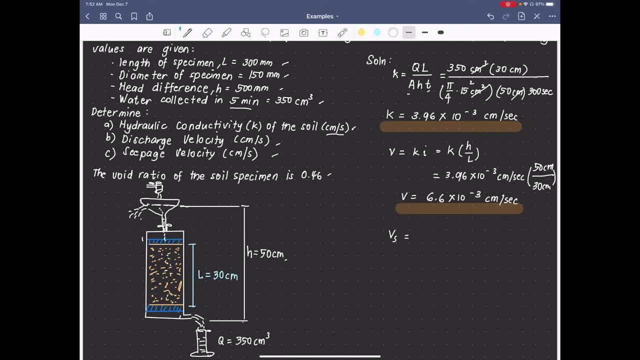 So this is a derived relationship between the sippage velocity and the discharge velocity that can be found in the book And that would be equal to V multiplied by 1, plus E divided by E. So this is a function of the void ratio. 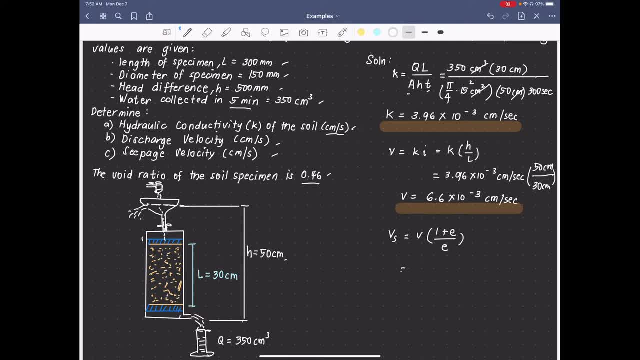 And the void ratio is given to be 0.46.. So from here we can solve for the sippage velocity, Which is equivalent to 6.6 by 10, raised to negative 3, multiplied by 1, plus a discharge void ratio of 0.46, all over 0.46.. 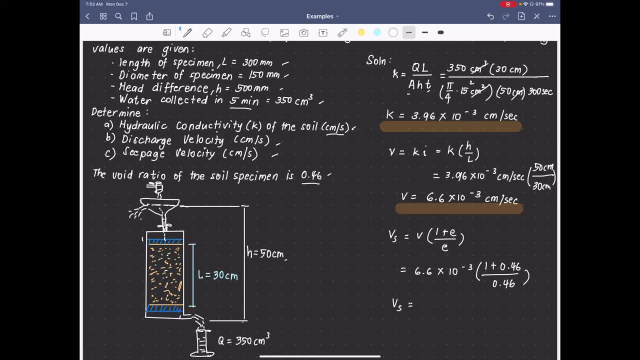 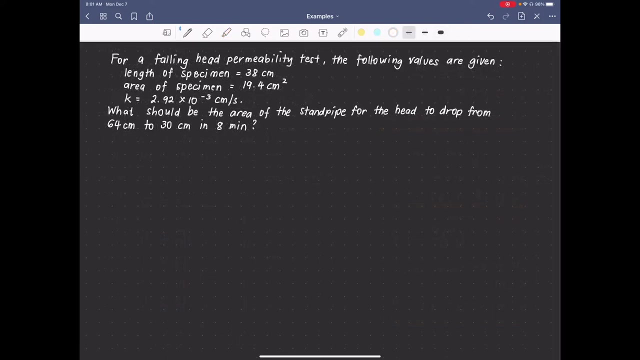 So the sippage velocity is equivalent to 20.95.. Raised to negative 3 cm per seconds. Okay, So that's how we calculate the permeability or hydraulic conductivity of fine sand. Now let's have another example, This time considering a falling sand. 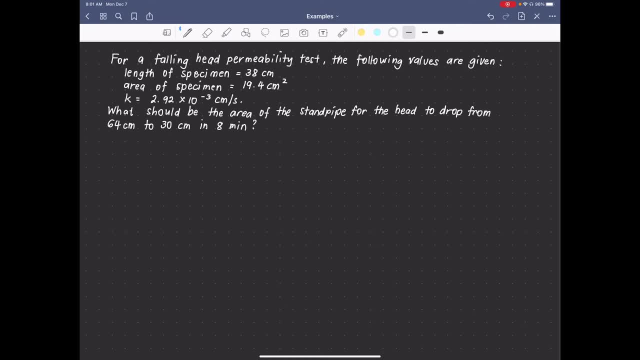 This time considering a falling head permeability test. So again, a falling head permeability test is applicable for fine materials or for silt and clay soil. So in this example, the following values are given: The length of the specimen is equivalent to 38 cm. 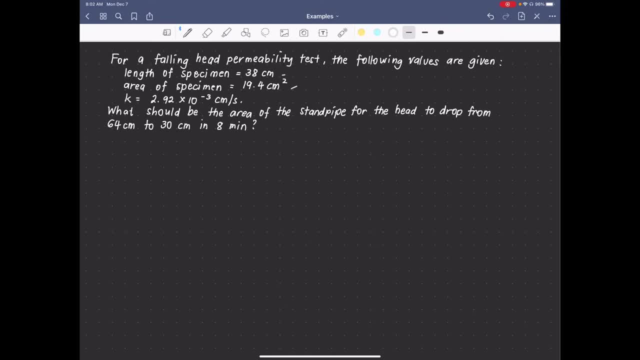 The area of the specimen is already given, So it's going to be 19.4 cm square. The permeability is known, Or the hydraulic conductivity value is 2.92 by 10 to the negative 3 cm per second. So what we are asked is the area of the standpipe. 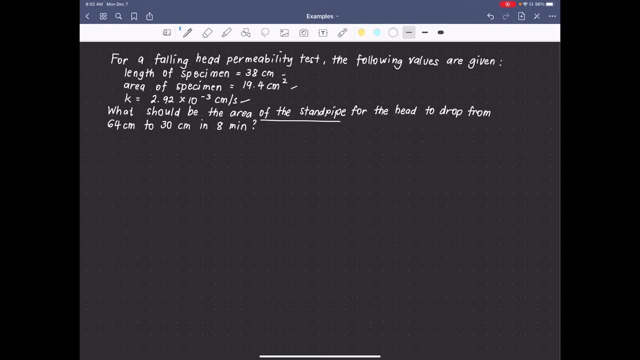 So this is the area of the standpipe, So that the head will drop from 64.5. Or CM To 30 cm Or centimeters in a span of eight minutes. So to give you the idea of the permeability test, or falling head permeability test. 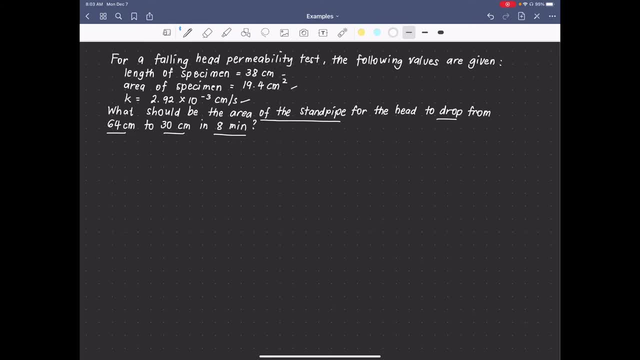 This is a different, a little different, with a constant head test, Because in the constant head test We have a constant head difference, but in the falling head test we have a different head difference at a certain time. so if you will look at the formula for the falling head test, the formula would be: 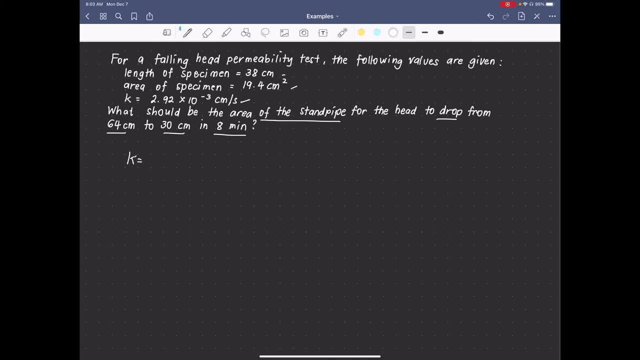 B 2.303 a by L, divided by capital A by T. this is log of this is base 10 H sub 1 divided by H sub 2. and B 2.303 a by L, divided by capital A by T. this is log of this is base 10 H sub 1 divided by H sub 2. 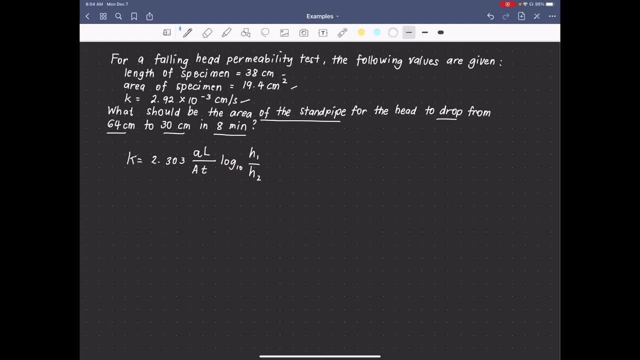 so if you look at the formula small a, here is the area of the standpipe. later we can see the standpipe. L is the length of the specimen. A is the area of the specimen which is similar to the constant head test. H1 is the head at time. T equals zero. 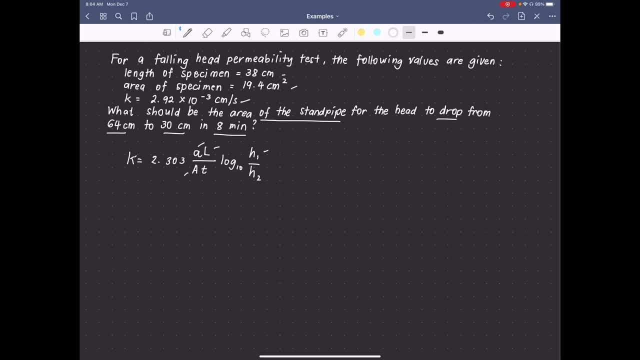 at the start of the test or at a certain time. t, which is known dapat, and H sub 2 is the head drop or the head difference at a certain period of time. so in this case it is 8 minutes. so let's look at the process for this falling head. 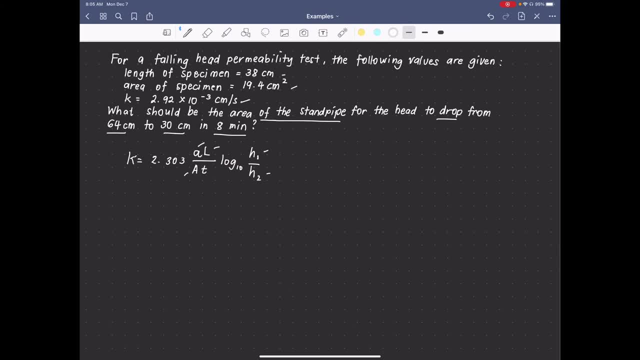 permeability test. so if we have similarly, we have the permeameter for the permeability apparatus, say here, and we still have our soil sample here- see here's our sample- and still have, oops, our porous stone here, we still have the outlet here so that water will be collected and 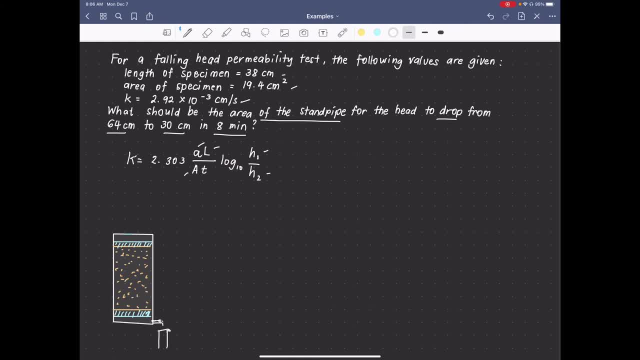 in a graduated cylinder, and this time we have a stand pipe here which is connected to our permeability apparatus. let me just enlarge a little our standpipe. oh sorry, okay, let us just enlarge a little. okay, this is standpipe, is connected to our faucet, of course, but we don't have a. 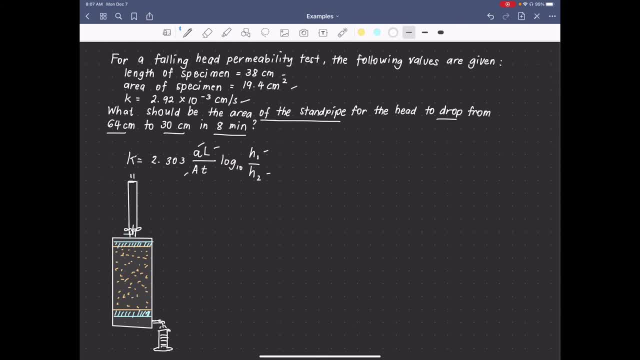 constant head this time. but this is, this changes okay, when we start allowing water to flow here and then water will get into our sample to pass through the porous stone, through our sample and to the porous stone at the bottom and it will go out to our outlet, to our graduated cylinder. 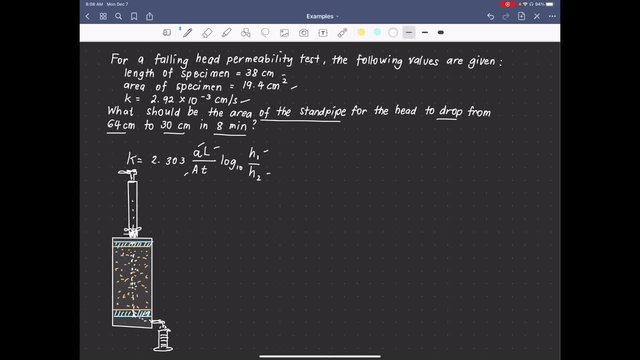 the same l. l is the length of our soil sample, which is here is equivalent to 38 cm. the area of the specimen is 19.4. so this is our capital, a, and then k is already given, okay. Okay, if we look at our formula, let's check. The following are known already: We have the length of the specimen. we have the area of the specimen time. t is 8 minutes, or this is equivalent to how many seconds. 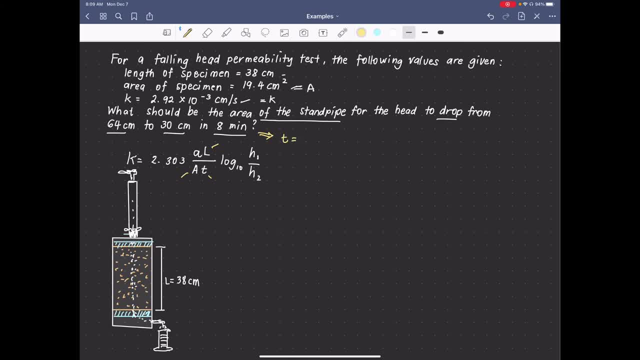 This is: t is equal to 8 minutes, that is, 480 seconds. so this is already known. This is known. k, this is unknown and h1 is known to be 64, and 64 centimeter and this is 30 centimeter. 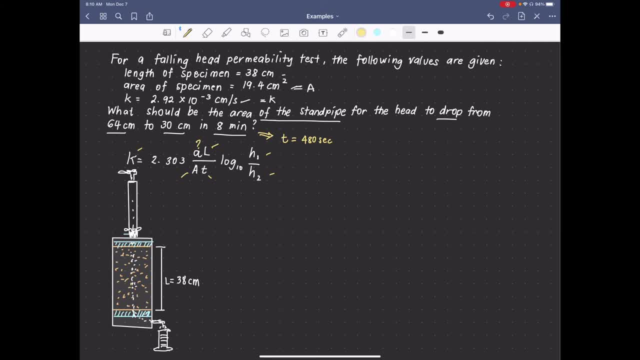 So we can right away calculate a. but just to make sure that we have the right answer, Just to give you an idea, on h1 and h2, or head difference 1 and head difference 2, that is when you start the test. let's say time is equal to 0, we will allow water to flow and when we start the test we have to measure a certain height from our standpipe. 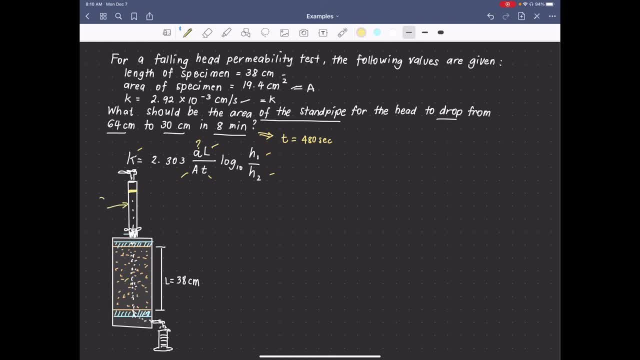 By the way, this is the area of the standpipe, that is A. that's the unknown. So here we have, from this point- let's say that's time equal 0, to our outlet, that is, our h1, which is equivalent to 64 centimeters. 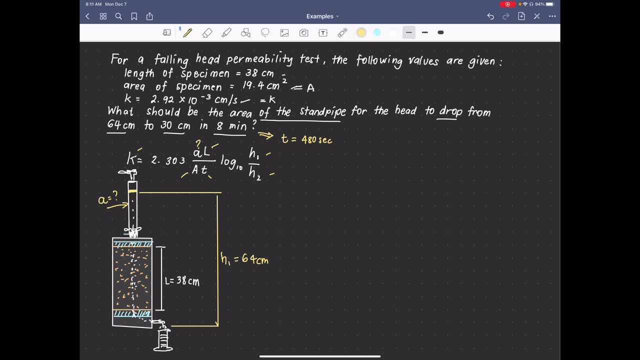 Now we have to stop water to flow from the faucet and allow the water to from this height, from 64 cm, allow the water to flow down to a certain height Within within 8 minutes, so say after 8 minutes. from this point, water goes down to this level from in our standpipe. 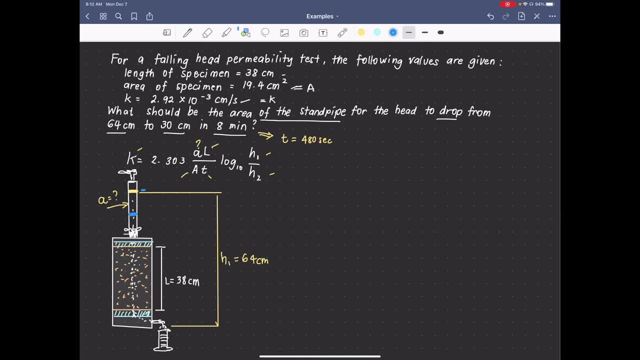 So from time equals 0 here to time equals 0 here, So from time equals 8 minutes again, the faucet is already closed. we allow water to flow from this level to this level and we get the height here, or the head difference, which is already given as 30 centimeters. 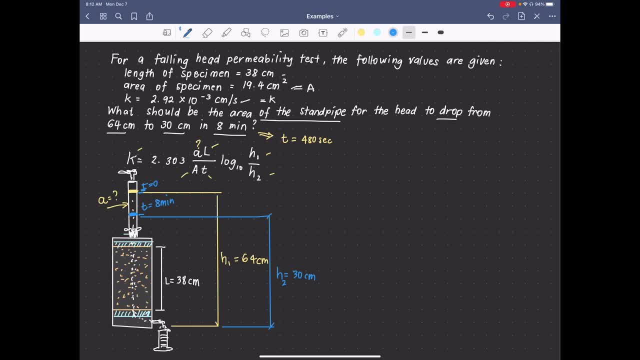 So from time equals. again, the faucet is already closed, we allow the water to flow from this level to this level and we get the height here or the head difference, which is already given as 30 centimeters. So that's the difference between the the difference of falling head permeability test, permeability test to the constant head test. 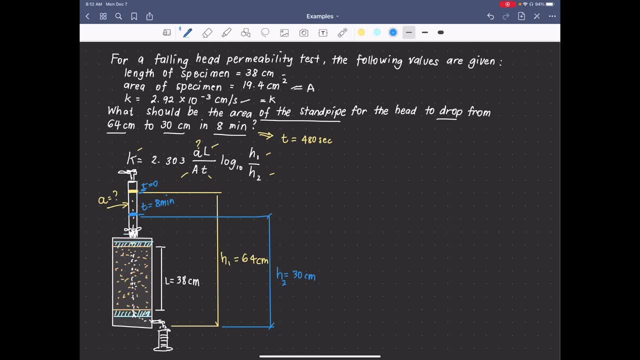 We don't allow water to continuously, continuously flow. Once the standpipe is already settled, we start water, we stop the water flow and we allow water to go down from the standpipe. Okay, So from here we can start the test.